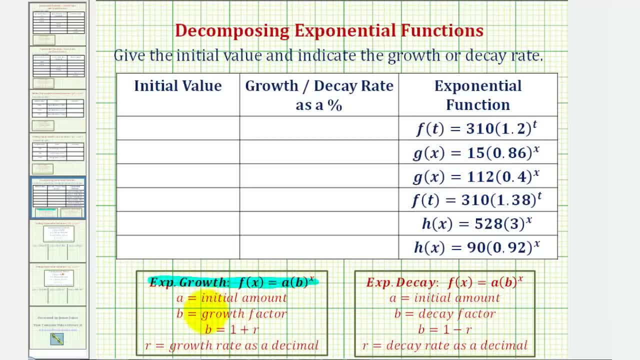 For exponential growth in this form. here the base b is called the growth factor, which is equal to one plus r, where r is the growth rate as a decimal. So because b is equal to one plus r, the base is always greater than one. 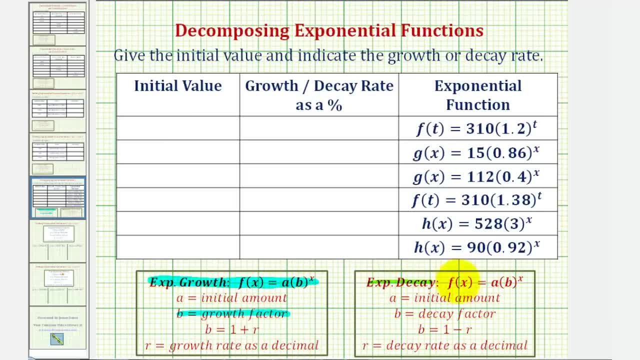 and therefore we have an increasing function. For exponential decay, the base b is called the decay factor, which is equal to one minus r, where r is the decay rate as a decimal. So because we're subtracting r here, for exponential decay the base is always less than one. 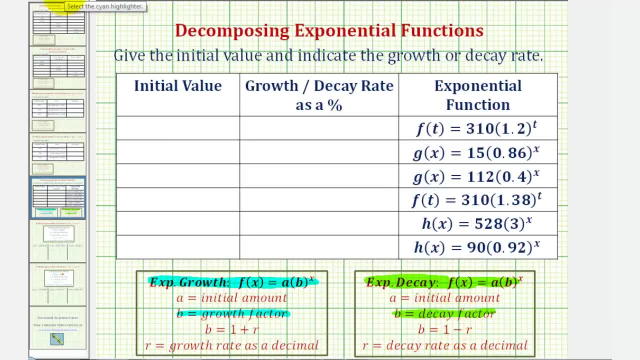 and therefore we have a decreasing function. So, looking at our six functions, notice how here the base is one point two, which is greater than one. So this would be exponential growth. Next, we have a base of zero point eight, six, which is less than one. 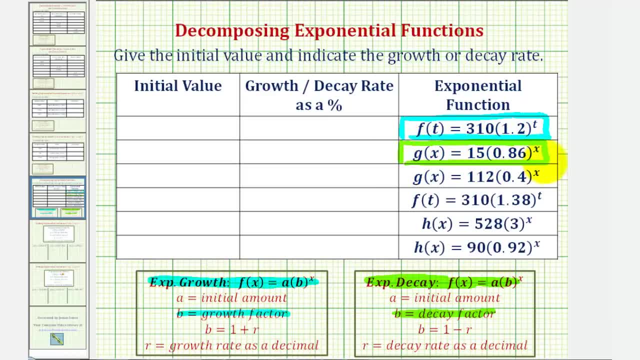 This would be exponential decay. Next, we have a base of zero point four. This is also exponential decay. Next, we have a base of one point three. eight, which is greater than one, So this would be exponential growth. Next, we have a base of three, which is greater than one. This is exponential growth. 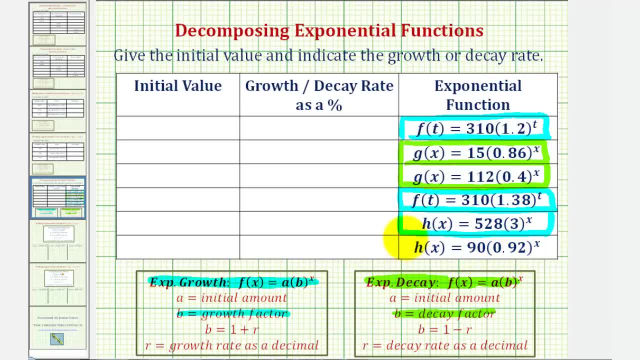 And finally, we have a base of zero point nine two. so we have exponential decay. Notice, in all these exponential functions, a is the initial amount or initial value which we can easily identify. So for this first function, notice how the initial value, initial amount, would be three hundred ten. 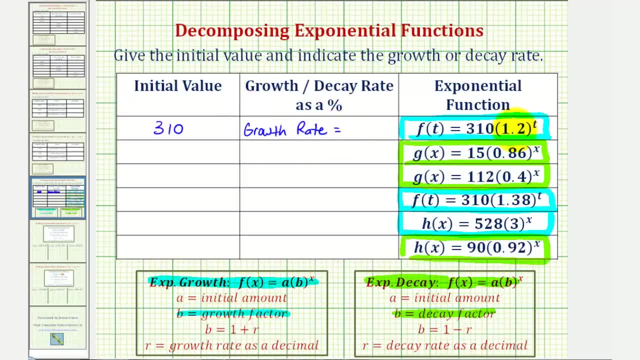 And now for the growth rate. we can find it using the equation b equals one plus r. since we know b is equal to one point two, We can probably determine this value mentally. but let's go ahead and show some work on the next slide. 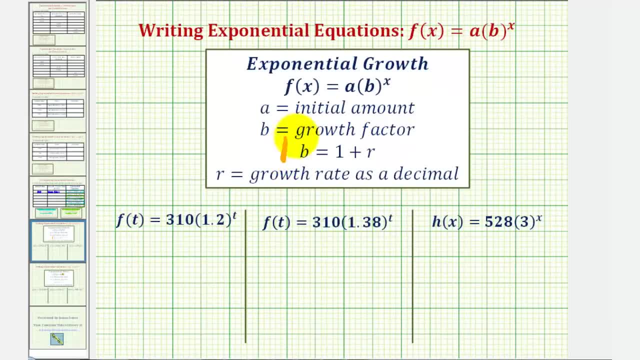 Again for exponential growth, we know that the base b, or the growth factor, is equal to one plus r, where for our first equation b is equal to one point two. So we'd have: one point two equals one plus r. 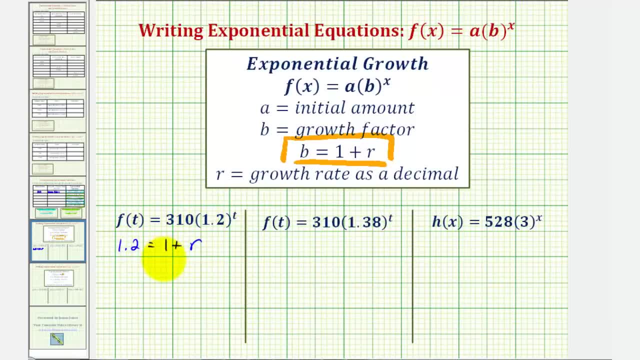 which, again, we can probably tell r must be zero point two, or we can subtract one on both sides, giving us r equals zero point two. So this is the decimal form of the growth rate, but we want this as a percentage, not as a decimal. 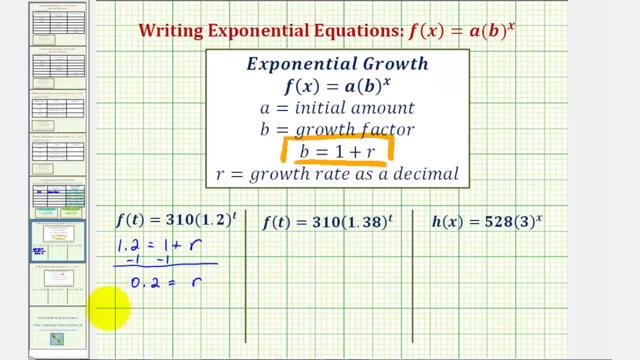 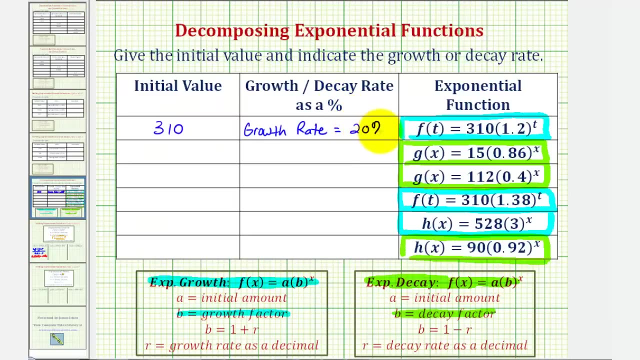 So to convert a decimal to a percentage, we multiply by one hundred and add a percent sign, which is equivalent to moving the decimal point to the right two places, giving us twenty percent. So for our first equation we have a growth rate of twenty percent. 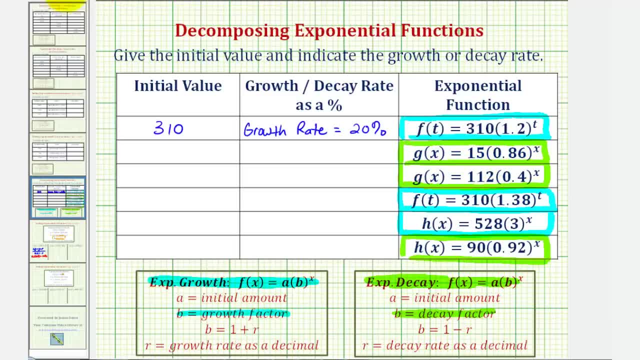 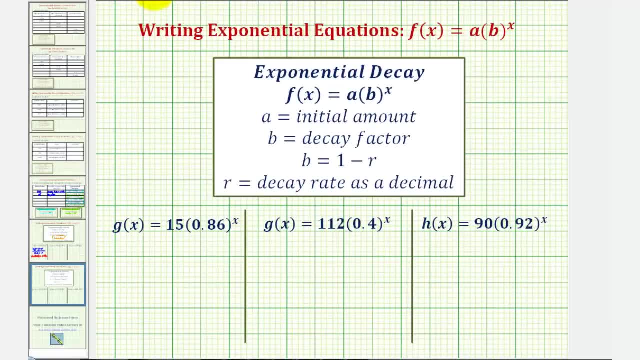 Our next function is exponential decay. The initial amount or initial value is still fifteen and that will show some work to find the decay rate. For exponential decay, the base b of the decay factor is equal to one minus r, where b is equal to zero point eight six. 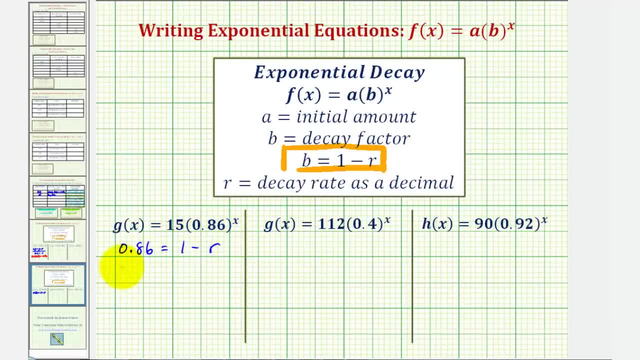 So we have zero point eight. six equals one minus r. Again, we probably can solve this mentally and recognize that r is equal to zero point one four. but if not, we can only solve this as an equation, Subtract one on both sides. 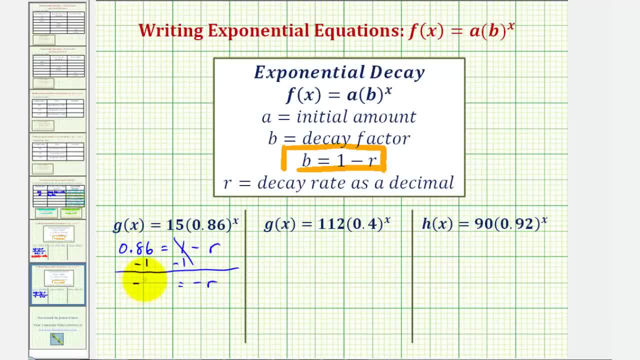 This would give us negative. r equals negative zero point one four divided by negative one and we have: r equals zero point one four. But this is the decimal form and we want the percent. so zero point one four times one hundred would give us fourteen. add the percent sign. 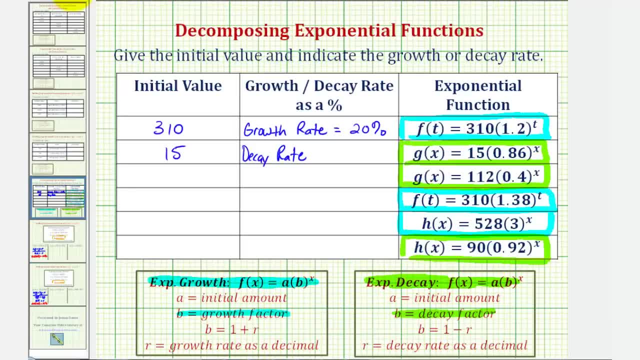 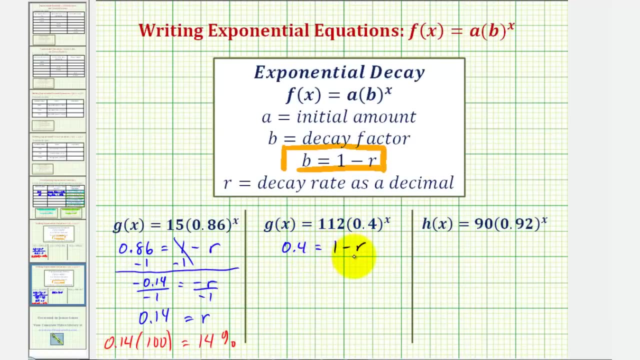 So we have a decay rate of fourteen percent. Next we have another exponential decay function where the decay factor is zero point four. So we'd have zero point four must equal one minus r. Again, we probably recognize that r is going to be. 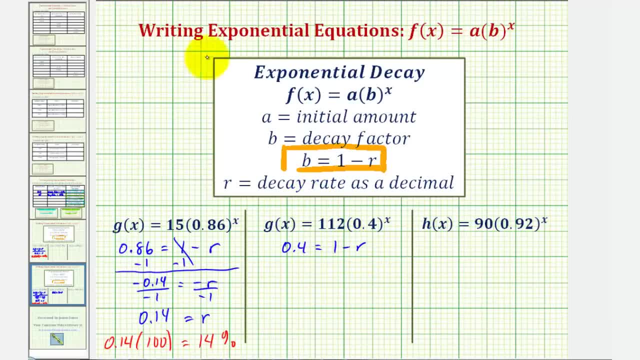 zero point six or sixty percent. but if we don't, we can show the work. Negative r equals negative zero point six. divided by negative one, We have: r equals zero point six, which would be zero point six times one hundred. 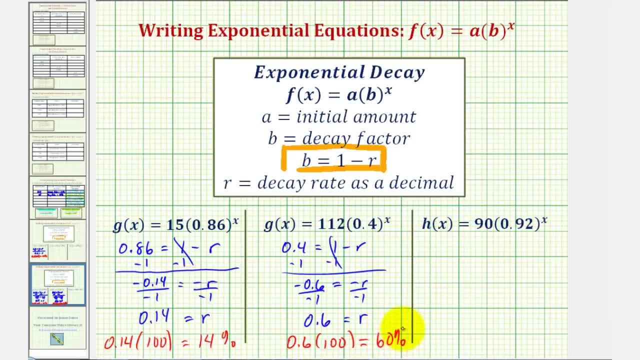 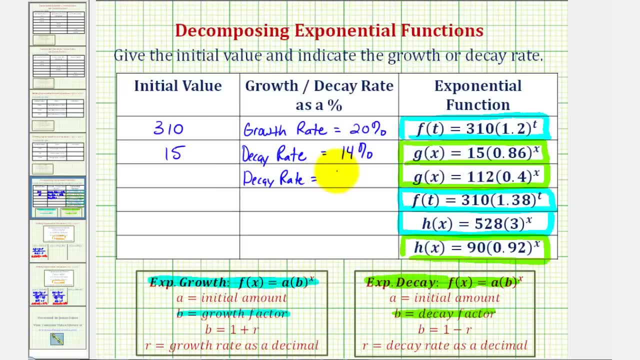 as a percentage, that'd be sixty percent. Notice how this is the same as moving the decimal point to the right two places. So our decay rate as a percentage is sixty percent and the initial value or initial amount is one hundred twelve. 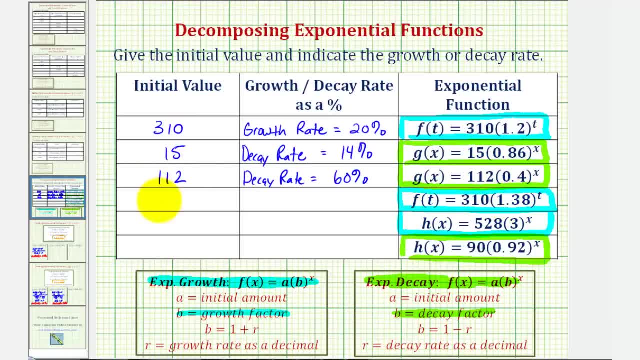 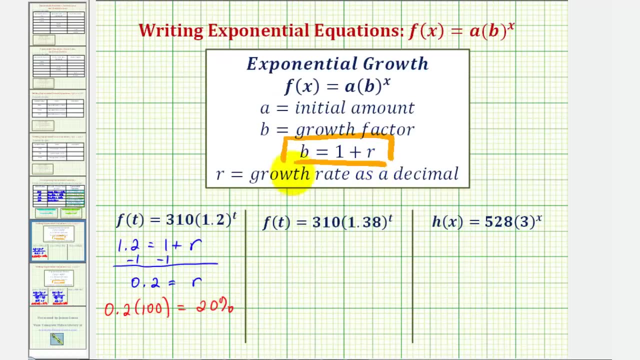 Our next function is exponential growth. The initial value is three hundred ten. so if b or the growth factor is one point three eight, we should be able to recognize that r would be zero point three, eight or thirty eight percent. But again, I'll go ahead and show the work. 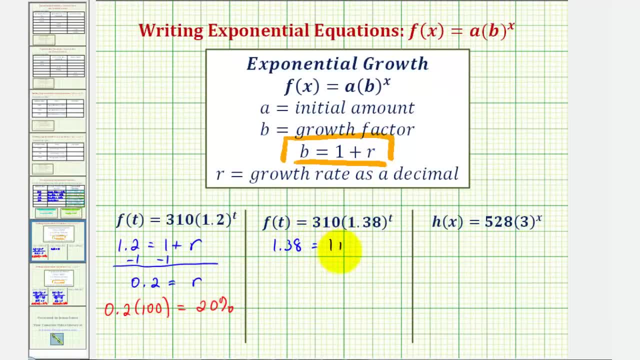 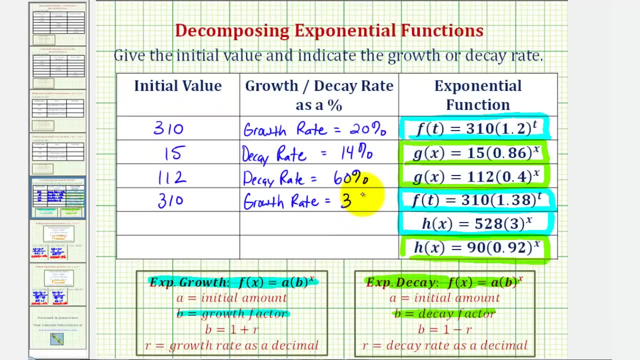 We would have one point three, eight equals one plus r. subtracting one on both sides gives us zero point three. eight equals r. zero point three, eight times one hundred would be thirty eight or thirty eight percent. We have another exponential growth function. 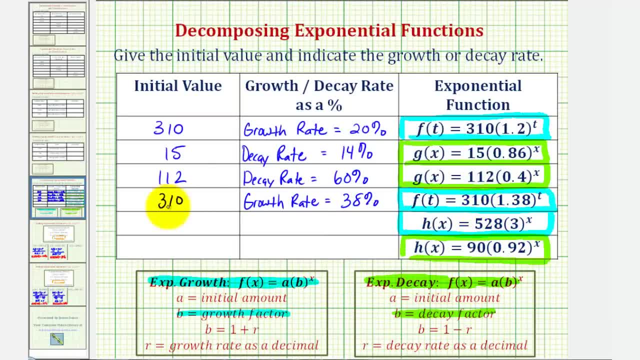 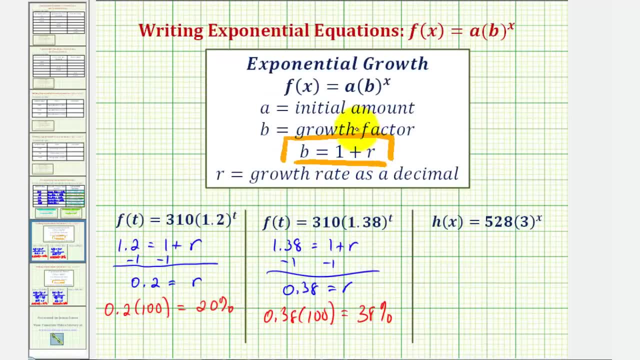 here. Well, the initial value is five hundred twenty eight. and let's go ahead and show some work for the growth rate. Notice how, if the growth factor or the base is three, we'd have three equals one plus r. subtracting one on both sides, we have r equals two. 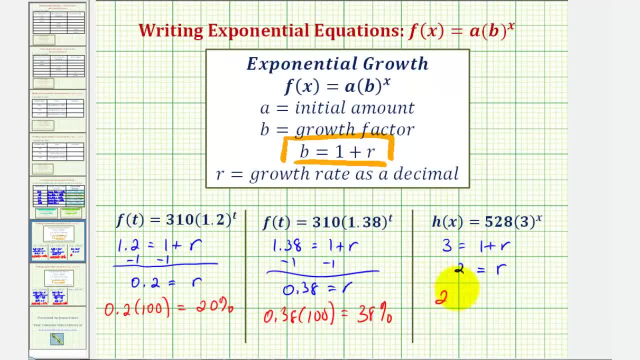 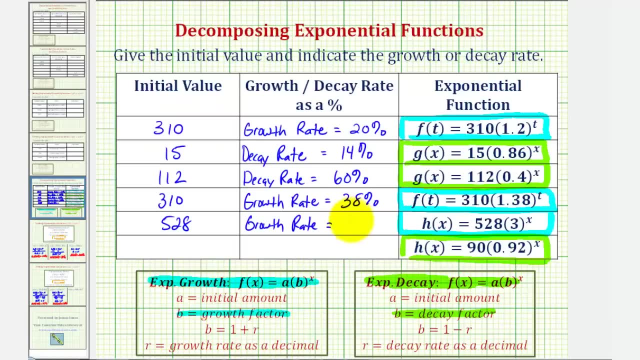 So the growth rate as a decimal is two. Well, two times one hundred is equal to two hundred or two hundred percent, which is our growth rate as a percentage. Our last function is exponential decay, with an initial value of ninety And the decay factor or the base b. 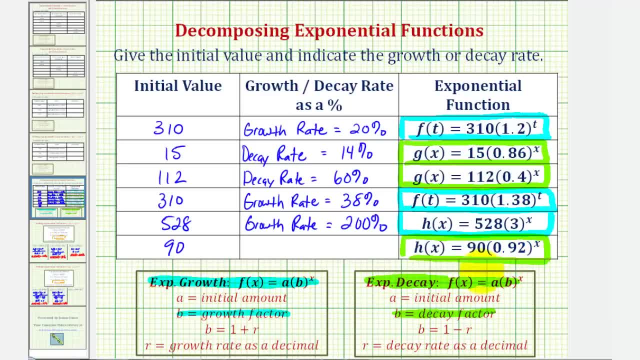 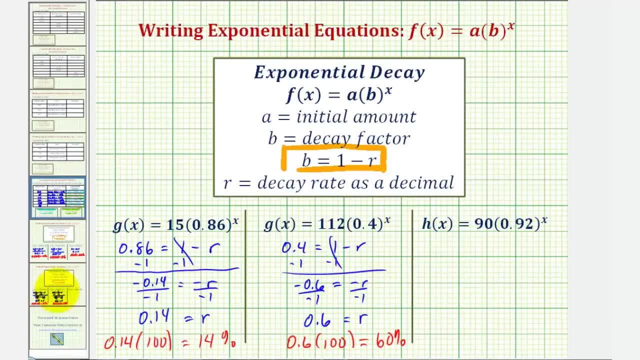 is equal to zero point nine two. So if we recognize that the decay rate is going to be point zero eight or eight percent, that's perfect. If not, we can show the work Where we'd have: b equals zero point nine two. 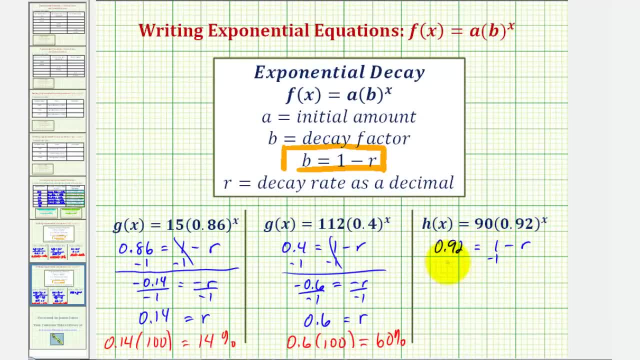 equals one minus r. subtract one on both sides, negative r equals negative zero point zero eight, and divide by negative one. So we have: r equals zero point zero eight as a decimal, as a percentage, multiply by one hundred, this would give us eight percent. 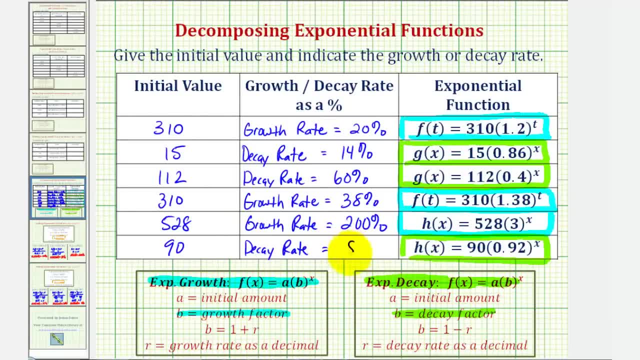 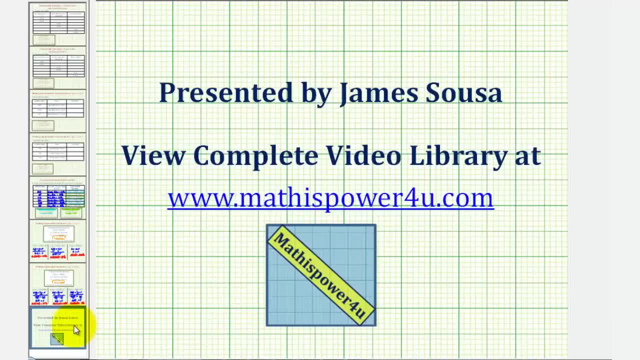 So our decay rate equals eight percent. I hope you found this helpful. Thank you.